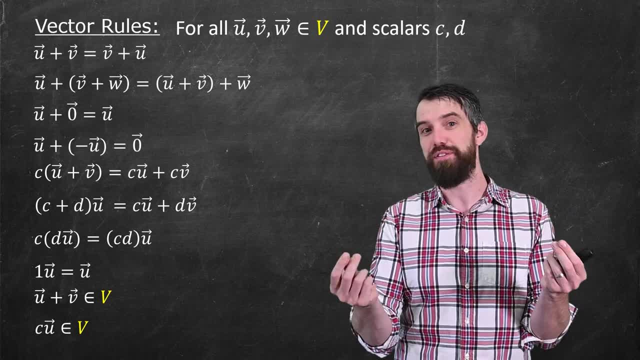 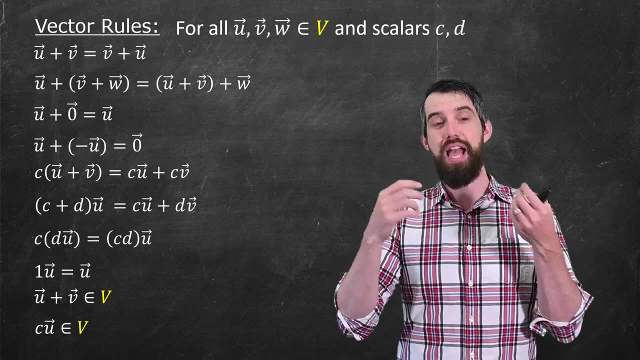 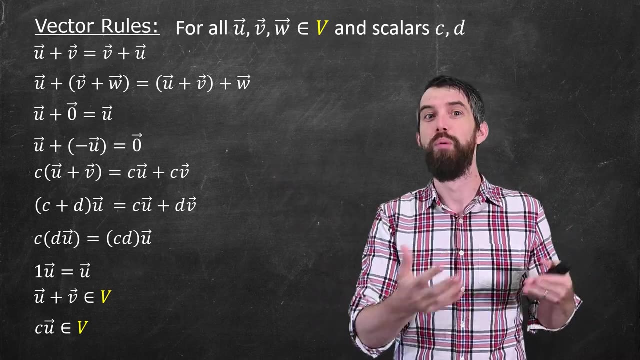 does as well. And indeed, whenever you have a mathematical object where there's a notion of scalar multiplication and a notion of vector addition that satisfies this long list of properties, all the rules that you would expect from normal study of the vector space of Rn, then we call that 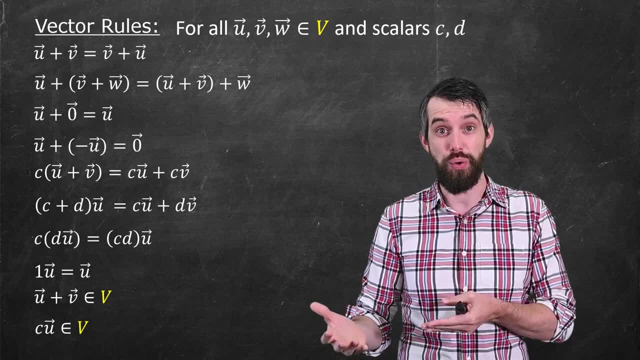 a vector space, And so, indeed, polynomials of degree less than or equal to 2 satisfy every one of these rules and are a vector space as well. So now we have the top-and-bottom linear dependence and independence span and finalization. 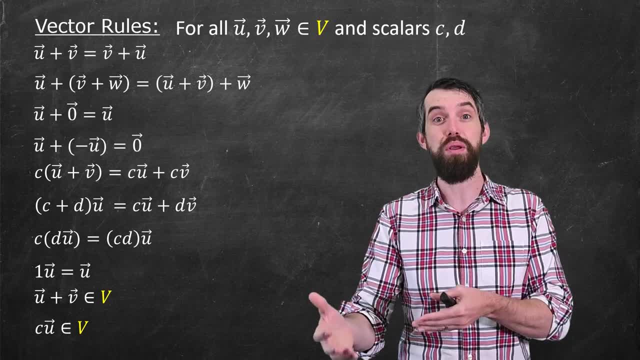 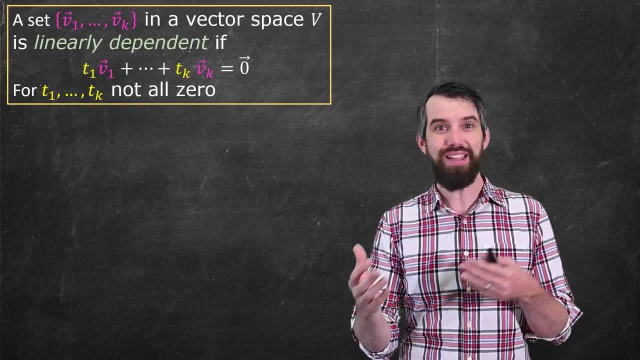 And, finally, basis in this new vector space of polynomials of degree less than or equal to n. First thing I'm going to talk about is linear dependence. The idea is exactly the same definition that we had for Rn, It's just said a little bit more arbitrarily. I'm going to begin with. 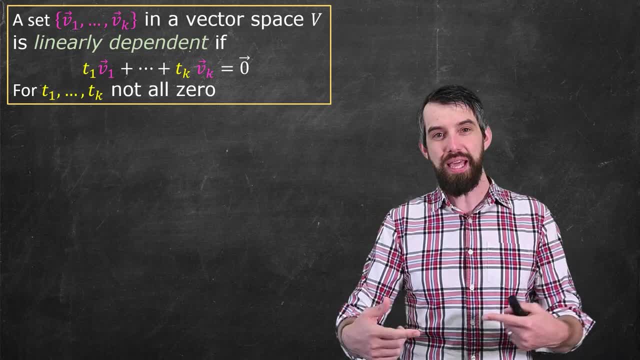 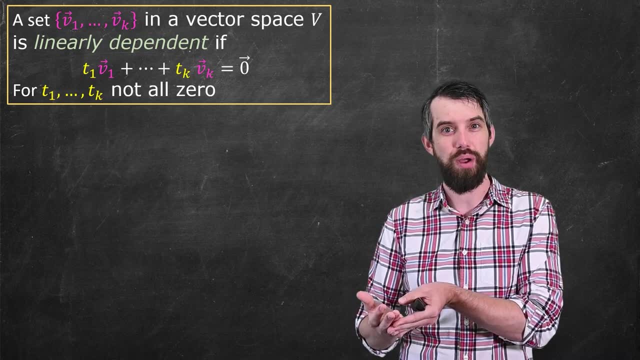 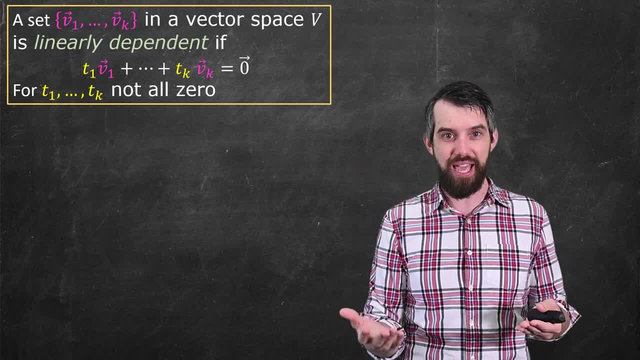 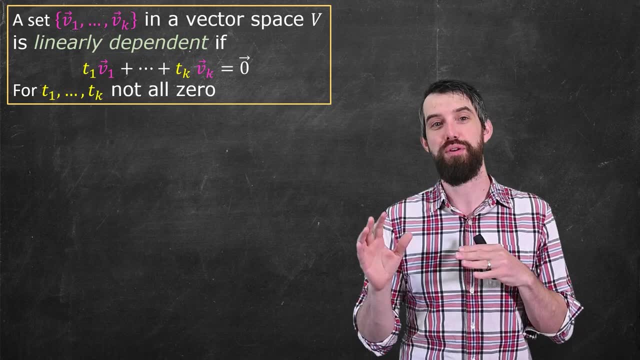 we've got a set of vectors, v1 down to vk, And then we've got a set of vectors and 0. That is, there's some t1 down to tk where the linear combination, where those t's are the coefficients that can add up to zero in a non-trivial way, with not all of those. 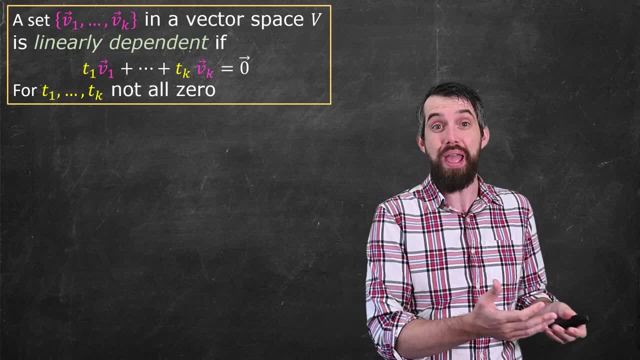 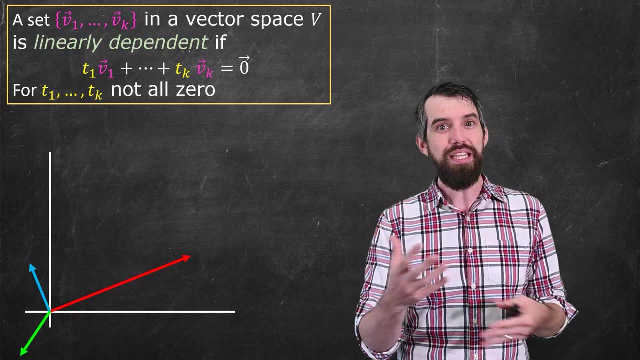 t's being zero. Now, if this was vectors in Rn, the familiar picture might be that, okay, I'll put up three different vectors living in, say, R2.. And then, by stretching these vectors and adding them tip to tail, I can rearrange these so that they form a loop. 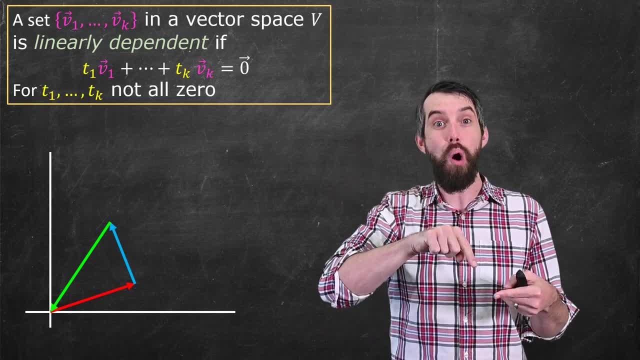 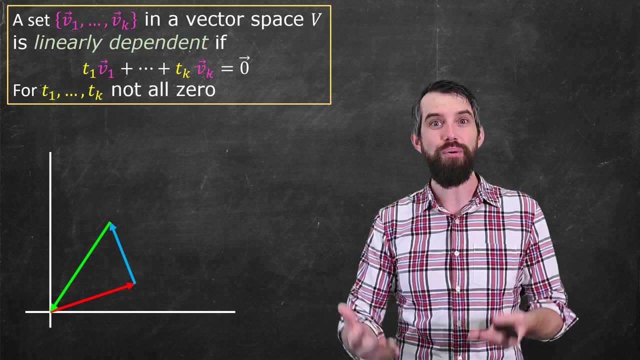 There's a linear combination of those three vectors so that when you add them up, they, they all come back to zero. That was the picture we saw when we were talking about, say, vectors in R2.. But the same general idea. 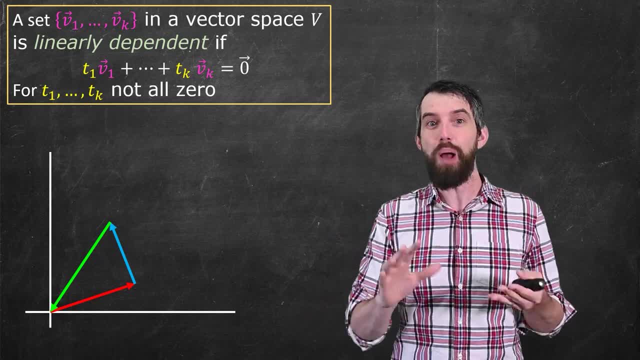 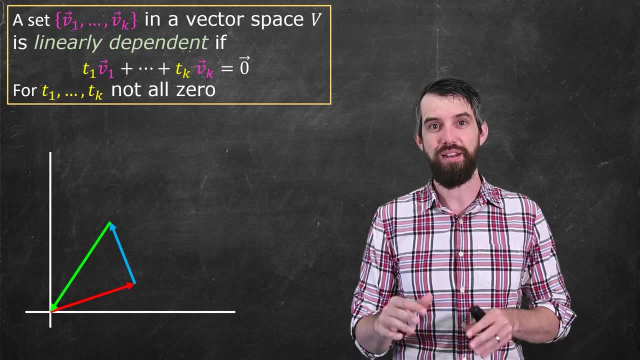 the same motivating definition is gonna apply even if we stop thinking about our vectors as being these things with arrows, living in R2, but instead being polynomials. It's the same definition. And then, likewise, if that's linear dependence, I can talk about linear independence. 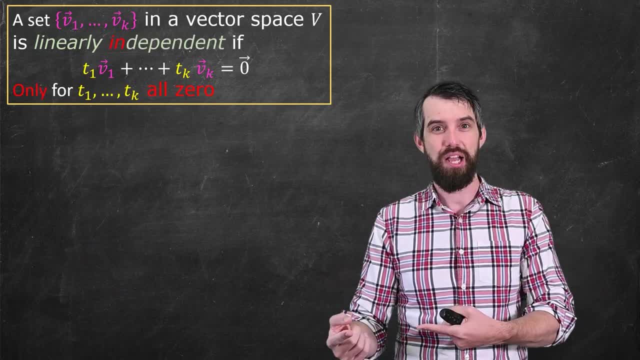 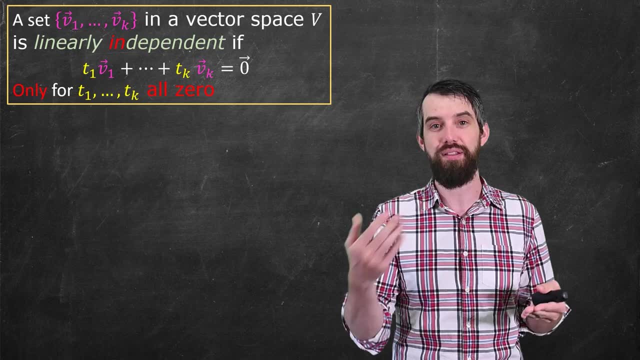 almost the exact same, It just says: well, the opposite is the case. The only way that the linear combination can be equal to zero is if all of the coefficients, the t1 down to the tk, are all individually zero, and that's linear independence. 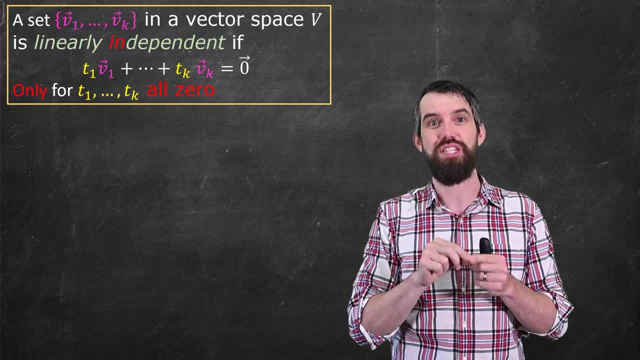 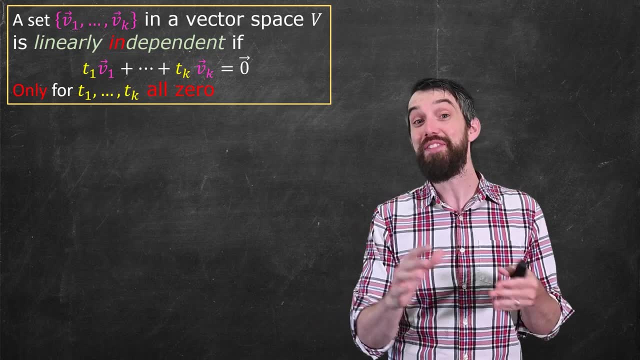 Basically says there's no way you can add up those vectors tip to tail that gets to zero, unless the length of all of them is set to be exactly zero by these coefficients. And so again we have to try to figure out what's that gonna mean in the context of polynomials. 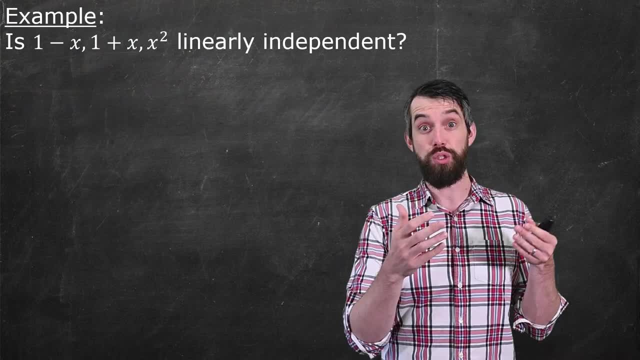 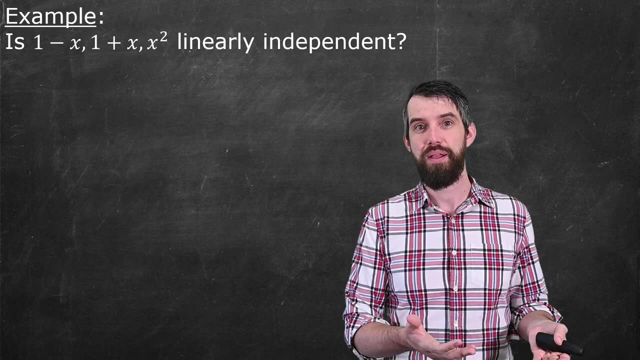 So let's see actually an example of this. I have the polynomials one minus x, one plus x and x squared. These are three polynomials and the question is: are they literally independent? What I need to do is take the linear combination. 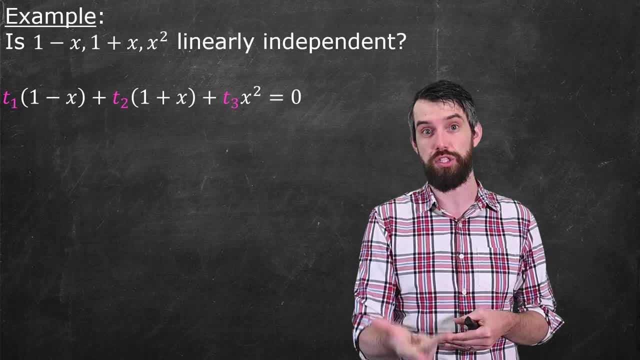 So I can take a generic linear combination. I have a t1,, a t2, and a t3, because there's three vectors and I multiply them to the one minus x, the one plus x and the x squared respectively, and I add this, equal to zero. 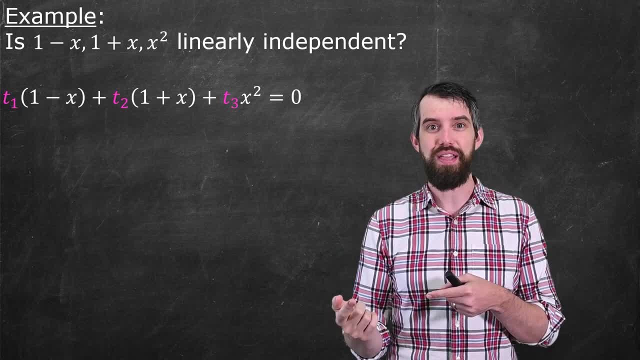 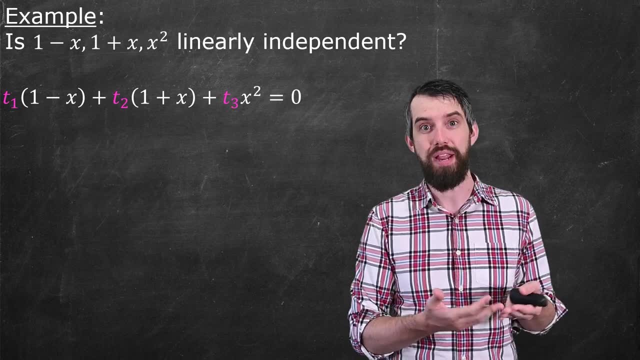 Now, how can I deal with this? One of the things that I observe is that in the one minus x and the one plus x, that there's a constant term in both of them- the one- and then there's a linear term. 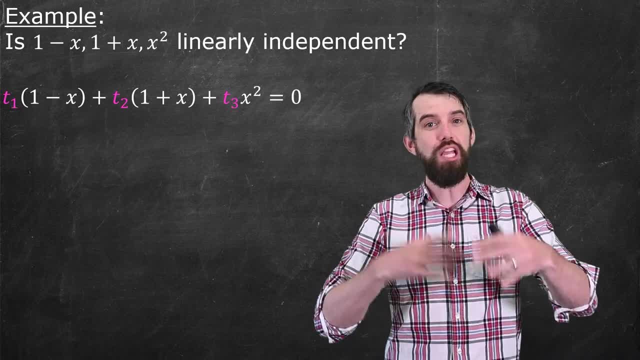 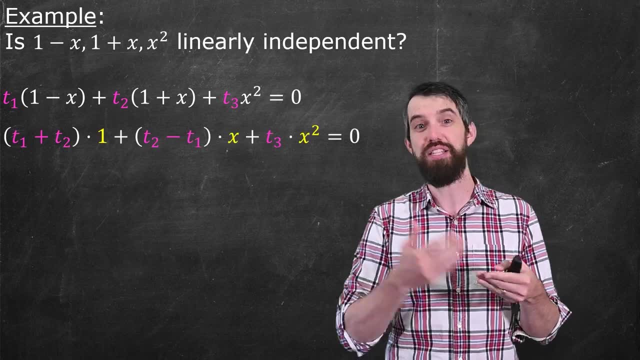 either the minus x or the plus x. So what I'm gonna do is just regroup this polynomial in terms of the powers of x. So what I mean by this is out the front. I'm gonna have a t1 plus t2,. 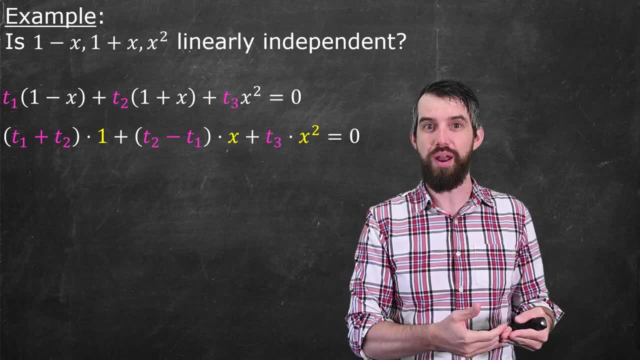 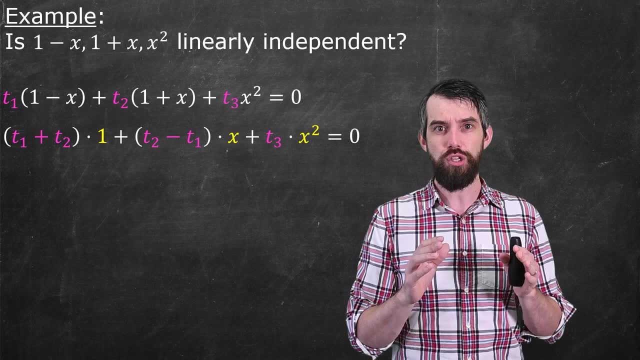 and it's just multiplied by one. Then I'm gonna have a t2 minus a t1, and it's multiplied by x and finally- I don't have to do anything here- The t3 is multiplied by x squared, and we're saying that equal to zero. 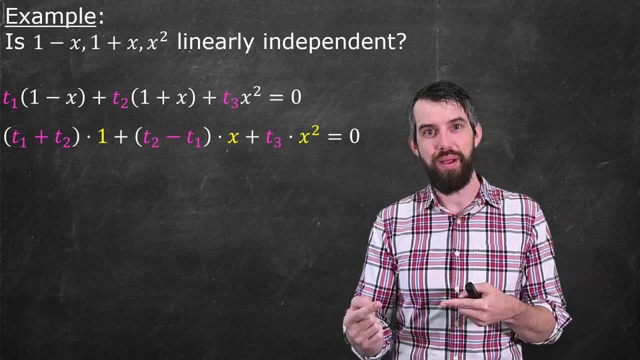 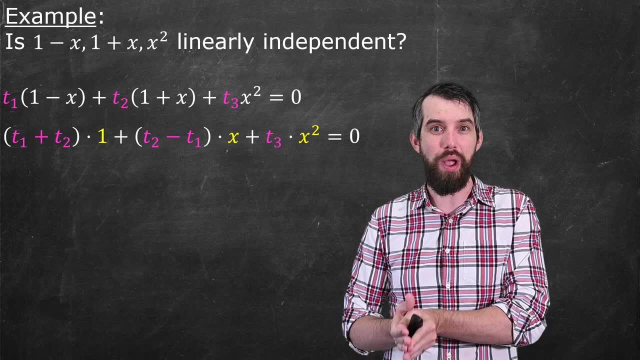 So what's different between these two lines is that in the second of them I've now ordered it, so it's a coefficient times one, a coefficient times x and a coefficient times x squared. One x and x squared are gonna be very special for us. 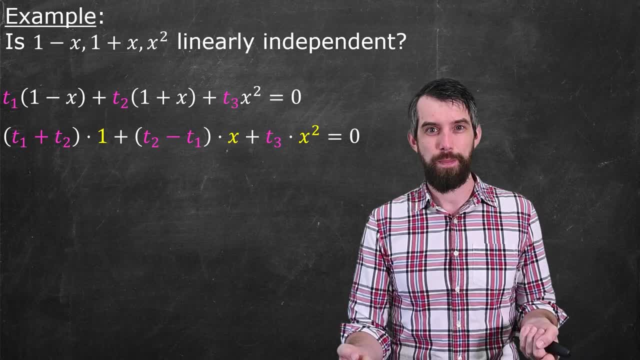 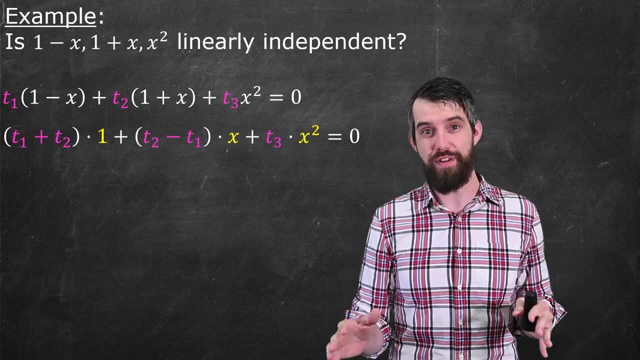 in a moment. so let's just put a pin on that Now. when I look at this equation, it's actually three different equations. The idea is that if this is true, it has to be true for all values of x. So, for example, if you set x equal to zero, 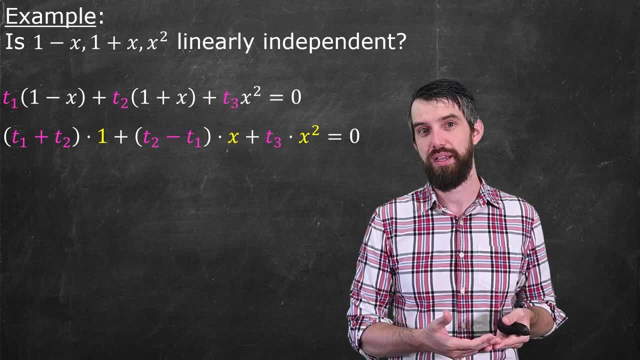 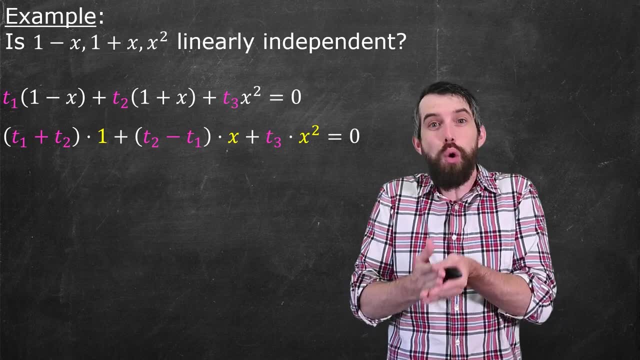 then only the constant term, the coefficient of one, would exist, And indeed, if you allow x to be multiple different values, it must mean that the coefficient of x is zero and that the coefficient of x squared is zero, And so this actually splits into three different equations. 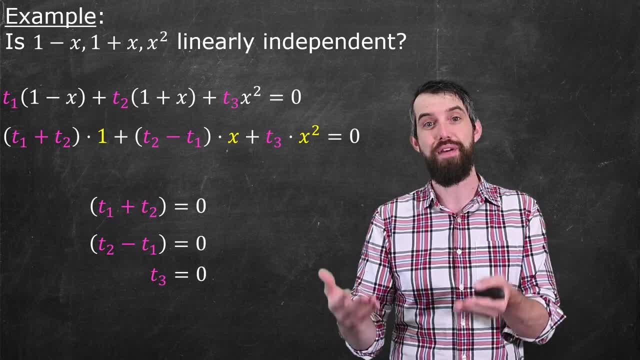 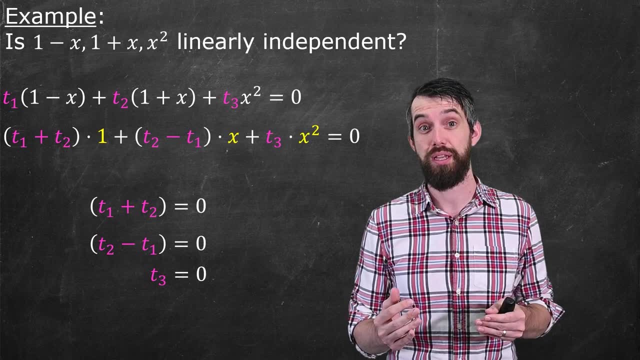 The first is for the coefficient of one, then the coefficient of x and then the coefficient of x, squared respectively, Because my x's are allowed to vary. this first equation is really just three different equations, But now this. that's something we've seen many times. 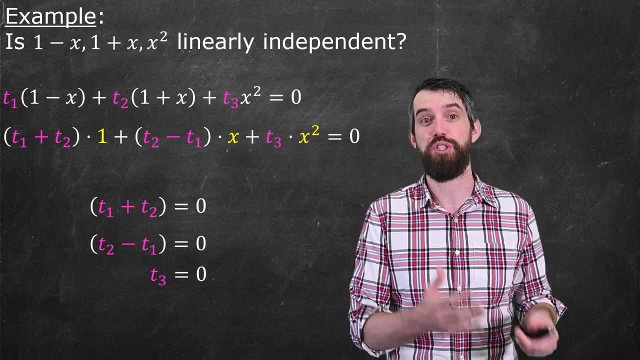 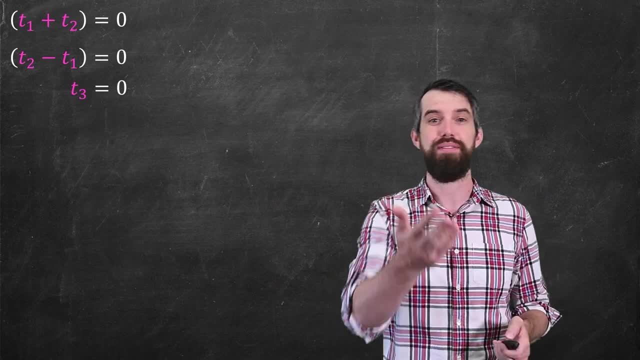 This is exactly the kind of system of equations we've studied extensively in our linear algebra course. So if I just focus on that alone, sort of blind to the fact that it began with polynomials, what would I do? Well, I'd say I could write down: 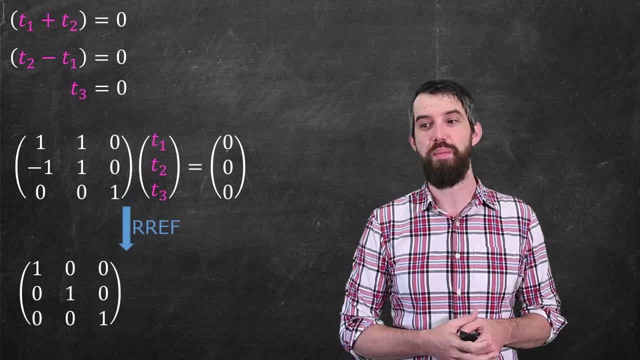 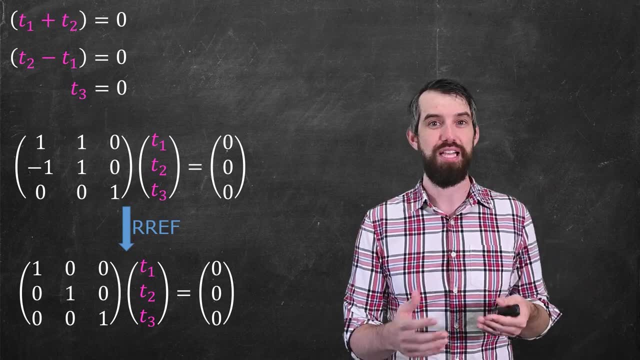 some sort of matrix for this. I'd say I could row reduce this particular matrix and I would just get that the identity matrix times t1,, t2, t3 is equal to zero. Now this identity matrix has full rank. It's got a one in every column. 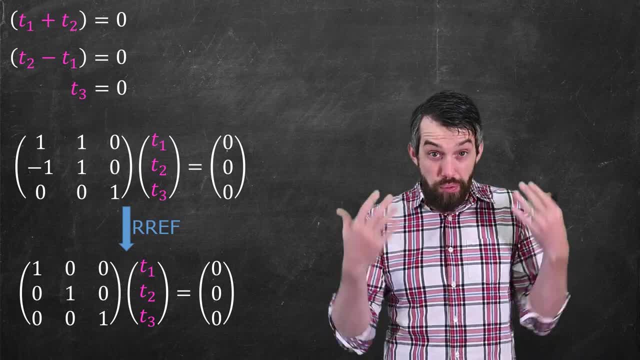 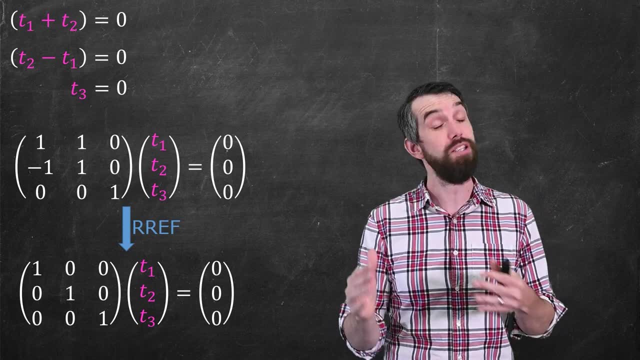 It's got a one in every row. There's many ways to say it. Either way, this is a unique solution. The only way to satisfy this is that t1 equals t2 equals t3 equals zero, And so this example is literally independent. 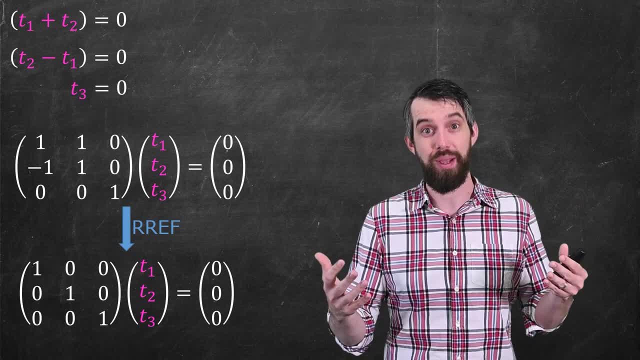 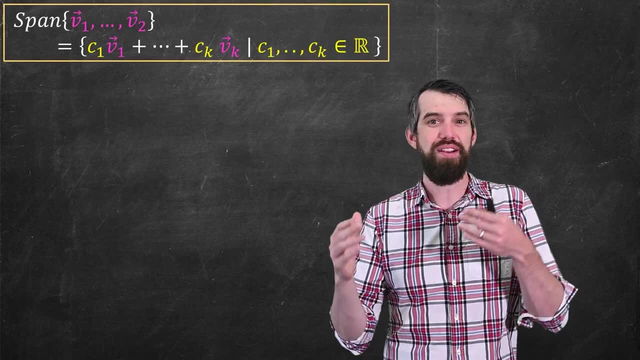 The only way you can satisfy this is that all of the coefficients are zero. It's literally independent. Okay, It's really independent. Next up, I'll talk about well, span. Span is actually defined just completely analogously to how we've done in the past. 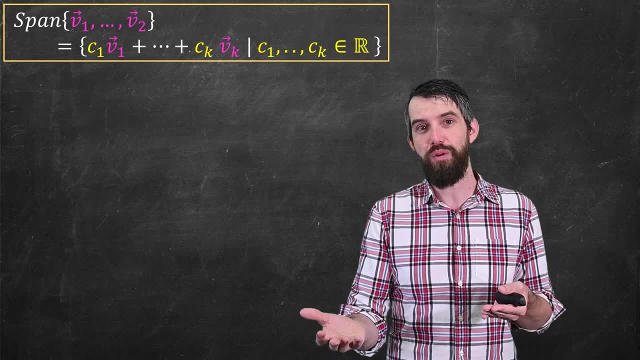 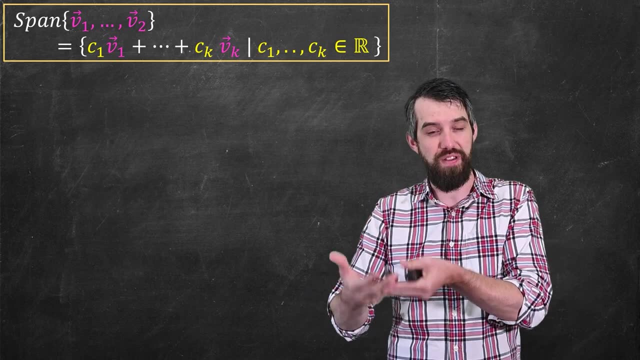 It says: if you want to take the span of a list of vectors, v1 down to vk, then what do you do? You just take all of your combinations of it. So now I'm going to write this as c1, v1 down to ck, vk. 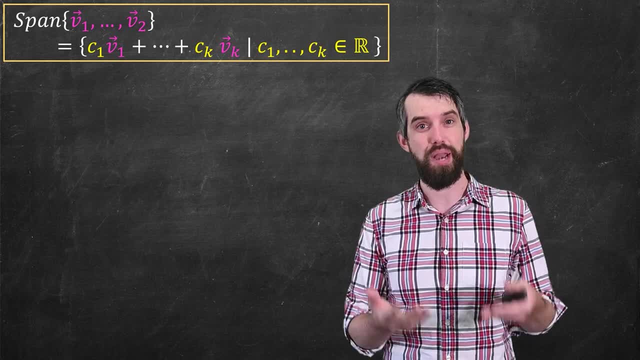 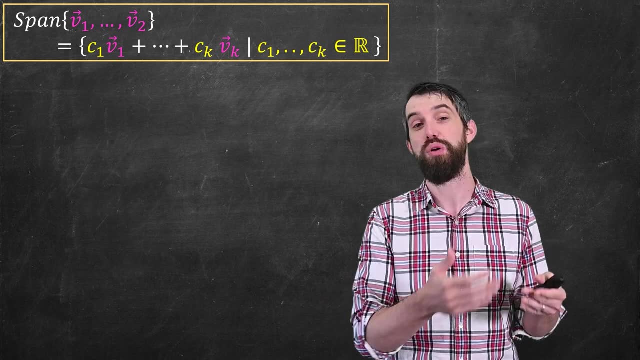 And my condition here is that those coefficients are just real numbers. By the way, the condition that just normal Rn and that polynomials of degree two with real coefficients both have the coefficients being real numbers. There's actually other generalizations of this. 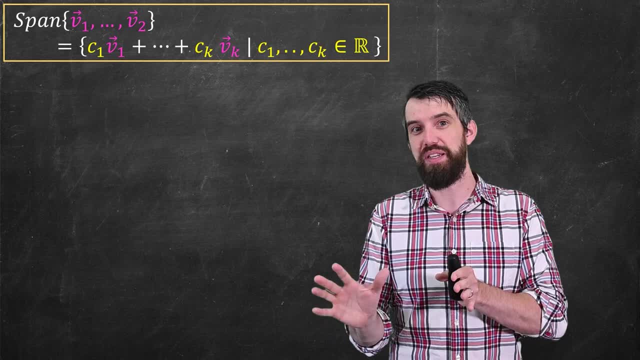 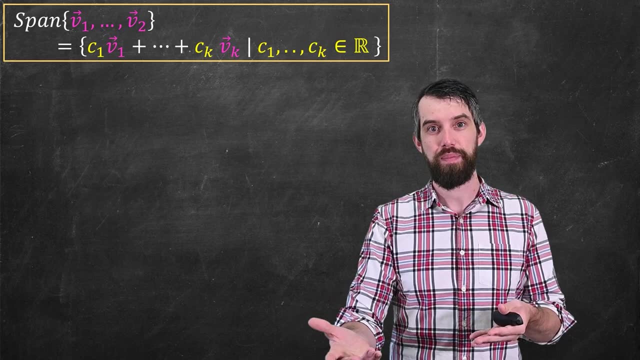 For example. you could imagine those coefficients could be complex numbers. There's other vector spaces that we're not going to talk about right now. Nevertheless, we have this notion of span. just says: take all the linear combinations and that's the span. 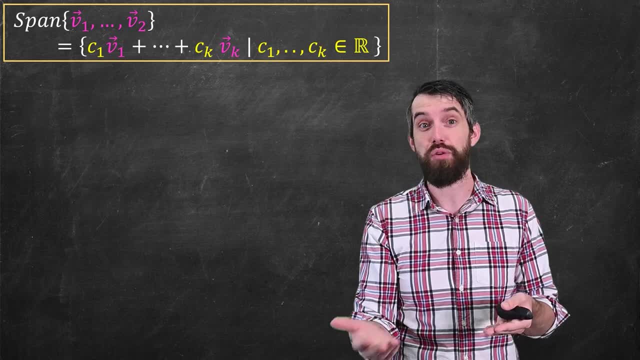 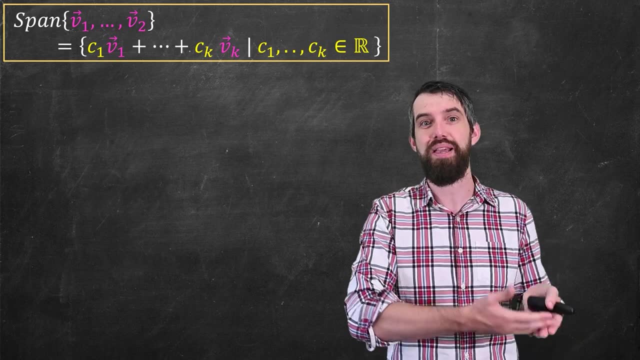 Many of the theorems we've proven in the past can just all be repeated. So, for example, the proof that the span is a subspace. you can repeat the exact same arguments and get that the span here is a subspace of the vector space of polynomial of degree less than or equal to. 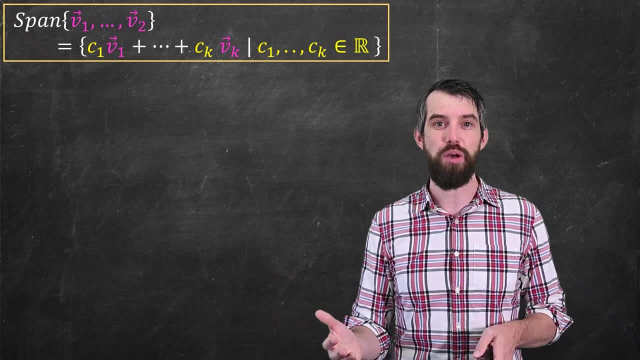 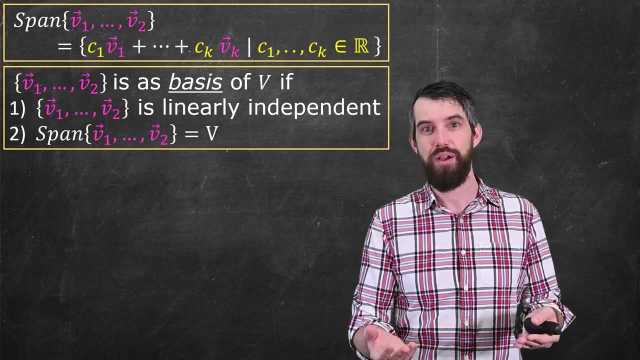 And then the final definition I'll put up is the notion of a basis. The notion of a basis, again, is exactly what we've seen before. It's just an arbitrary vector. space V now, which in the examples we're going to talk about. 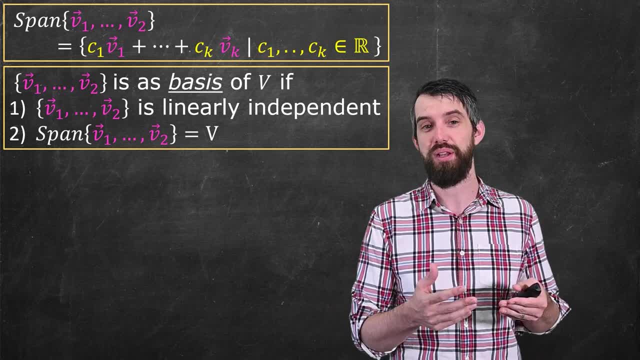 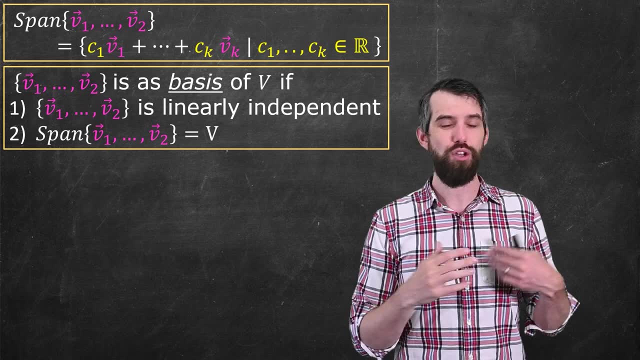 is often going to be polynomials of degree less than or equal to n in the real numbers. Nevertheless, it's got the two conditions: one, linear independence, and two, that it spans the vector space. So if I ask you to prove something as a basis, 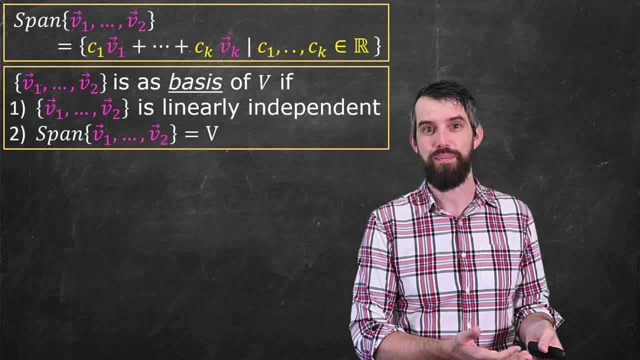 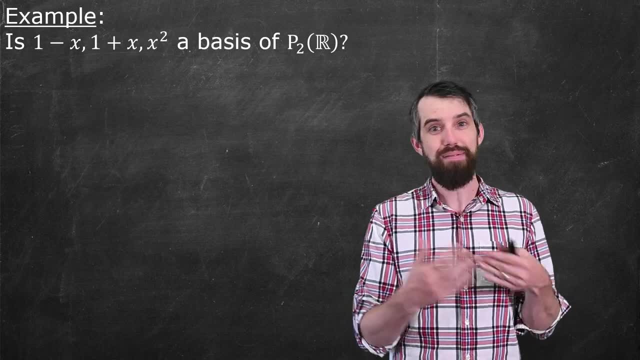 you basically have these two different things: you have to check linear independence and span. Okay, so well, let's do this Same example that we had previously, namely the 1 minus x, 1 plus x and x squared. Now I've just changed the question. 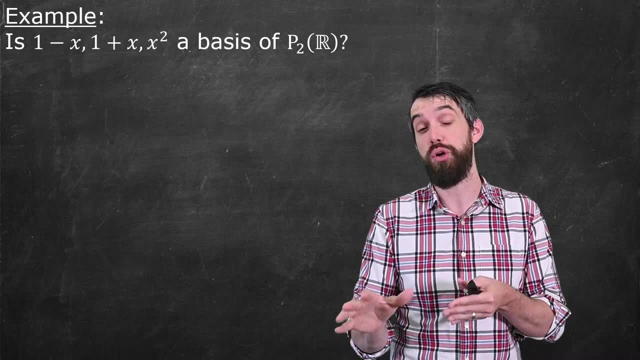 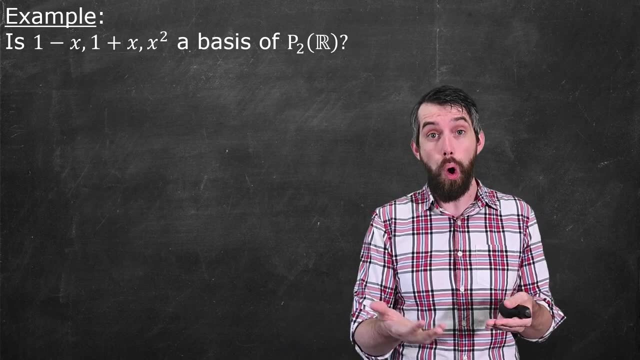 I'm saying, is it a basis? Well, we've already done a lot of work on this example. We've already shown that that list of three vectors is linearly independent. So what remains to show that it's a basis is that it spans all of the two degree polynomials. 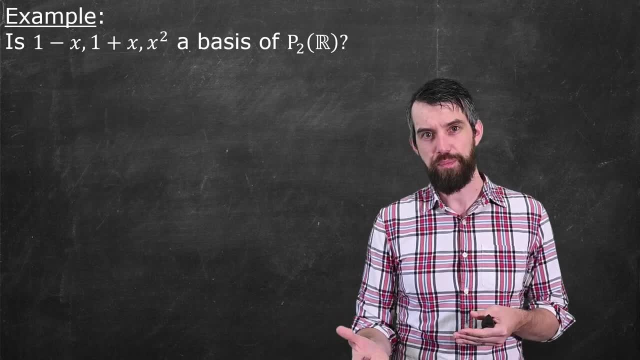 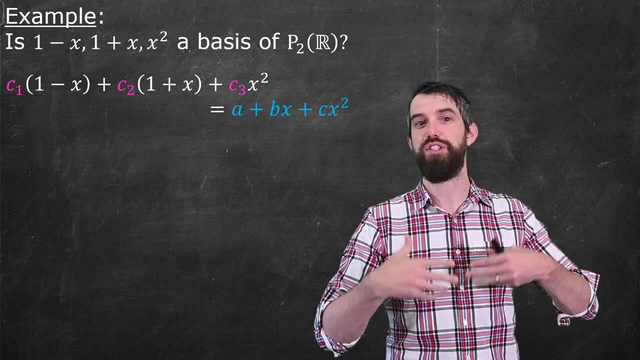 p2, over the real numbers. So what does that mean? Well, what I'm saying now is, if I take all linear combinations- note that I'm just shifting notation to match my definition- My coefficients are now c1,, c2, and c3., 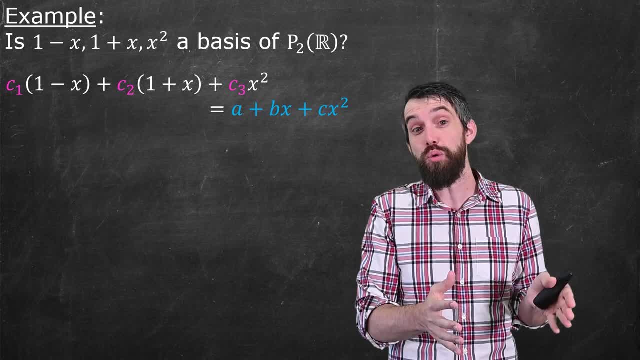 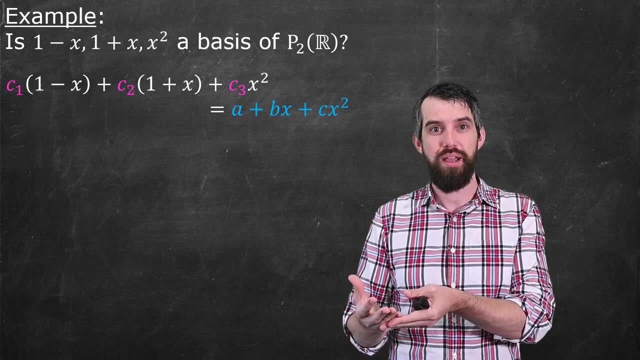 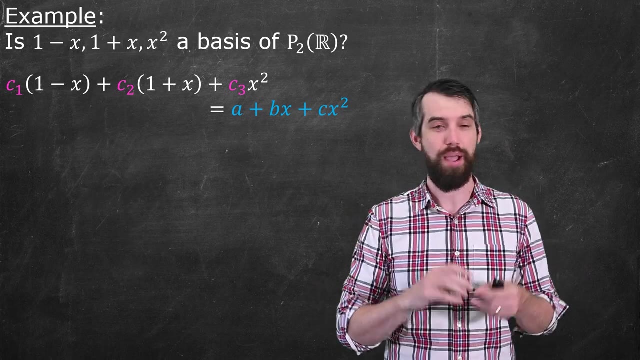 But nevertheless it's the exact same expression. but I'm saying that this equals not zero now, but an arbitrary polynomial: a plus bx plus cx squared. And the point is, could I take a linear combination of the three given vectors and get to anything with any value of a, b and c? 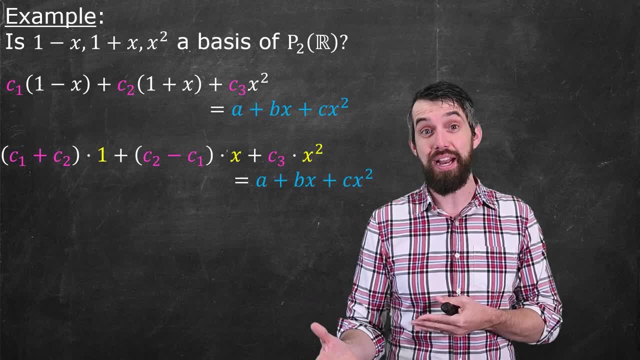 I'm going to rearrange in exactly the same way. so the left-hand side is well a coefficient in front of 1, a coefficient in front of x and a coefficient in front of x squared, And then we're going to do this: 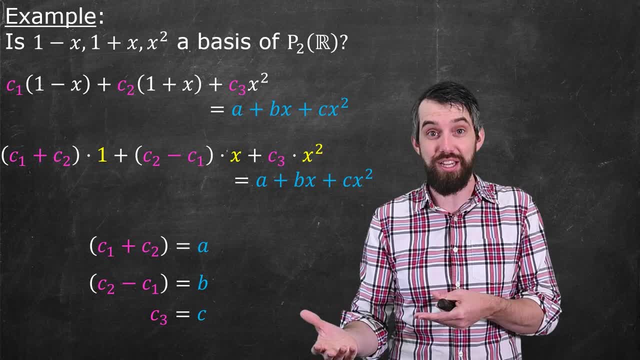 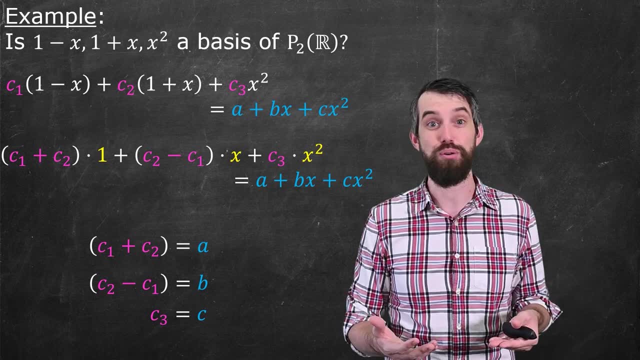 And in the exact same way, I can go and interpret this as three different equations: the equation that has to do with the coefficients of 1, the coefficients of x and the coefficients of x squared, The only difference now as opposed to the right-hand side, being 0, 0, 0,. 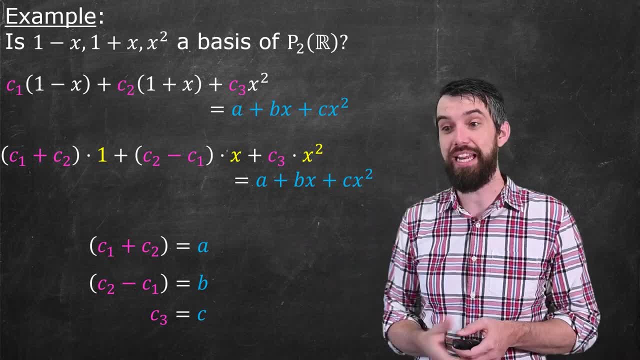 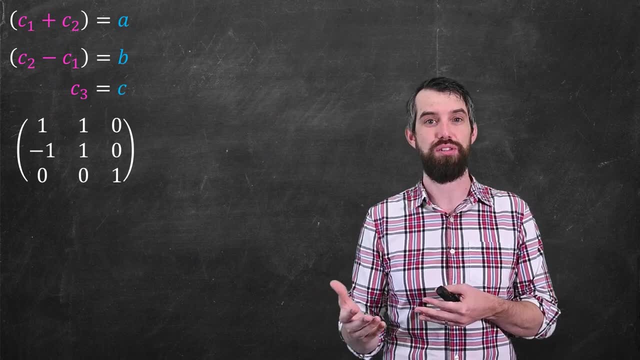 it's now a, b, c. OK, so, focusing in just on this system of equations, it's exactly like we've seen before. The coefficient matrix on the left-hand side just looks exactly the same as it did previously. I can row, reduce it in exactly the same way. 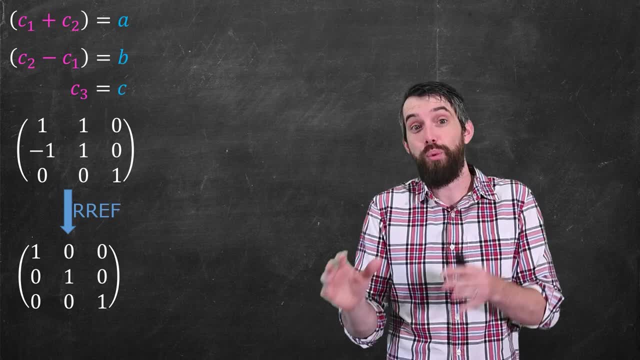 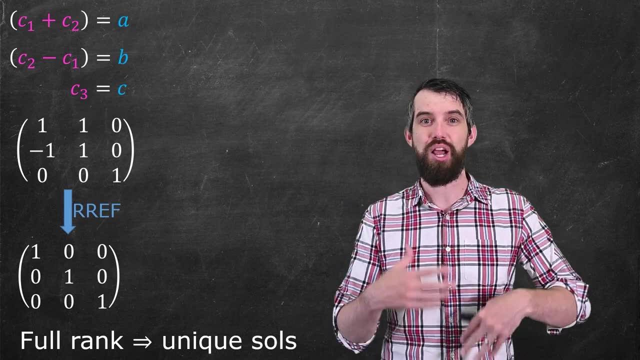 and I get the identity matrix. And because I have this identity matrix with its full rank, it means that every ax equal to b gives a unique solution. Or in other words, this original system that I have. does it matter what your little a, your little b? 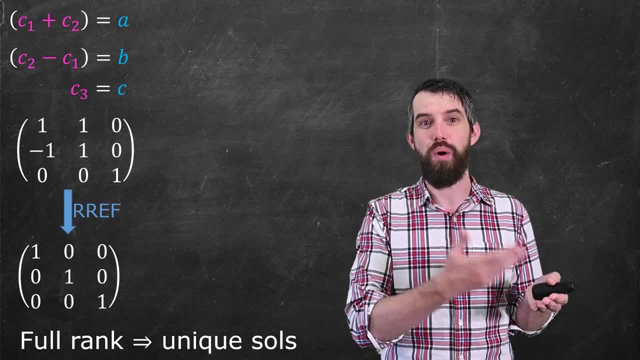 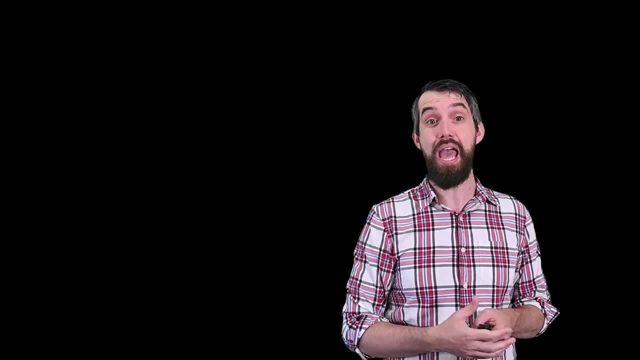 and your little c was you could always find the coefficients c1,, c2, and c3 such that it satisfies it. This is going to always be solved, And so, for our example that we have, it matches both conditions. It's got the linear independence. 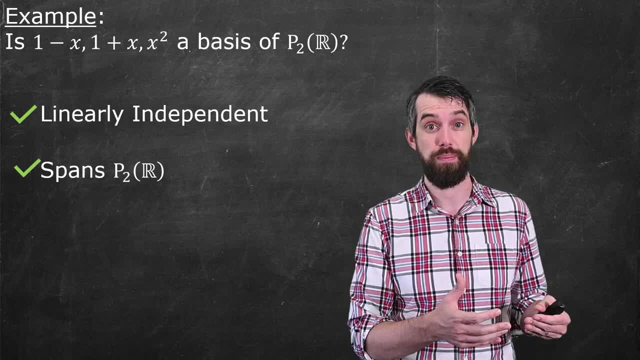 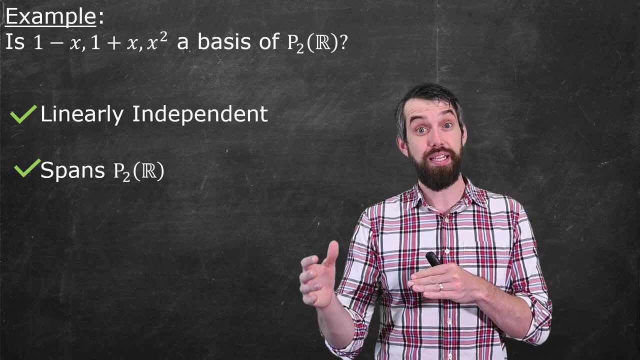 and it's got the fact that it spans all of the degree two polynomials. So, yes, this is a basis for this particular vector space. Now, while it's true this is a basis, it is not what I will call the canonical basis. 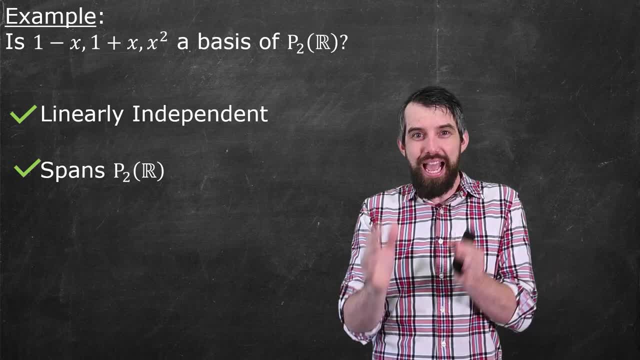 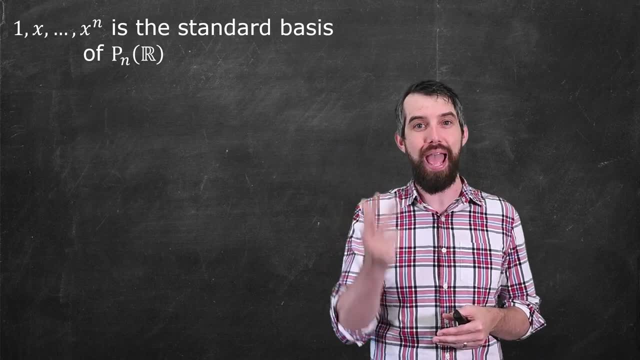 or the most natural basis for you to use. The most natural basis is: well, we've actually almost seen it already. It's the one: the x, the x, squared, dot, dot, dot all the way down to xn. 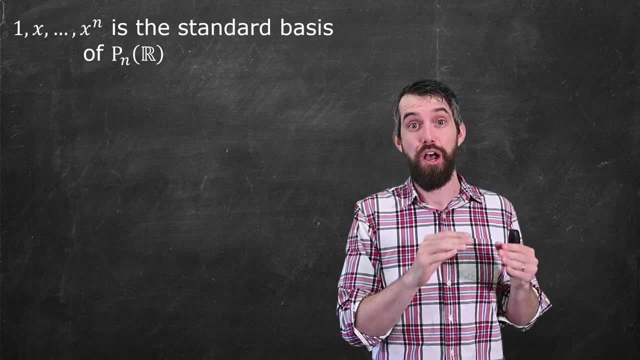 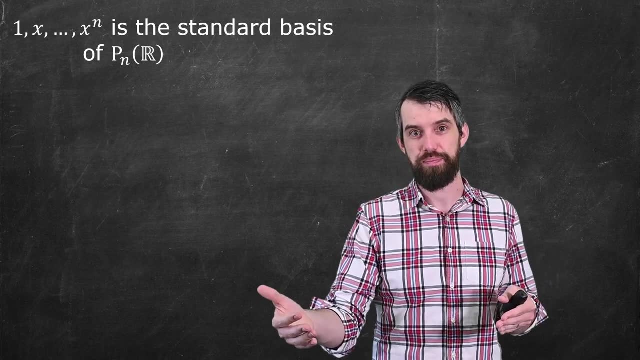 That is, the so-called canonical or standard basis for Pn of, or, in other words, the polynomials of degree less than or equal to n and over the real numbers. And indeed, to illustrate this well, we'll just repeat the computation. 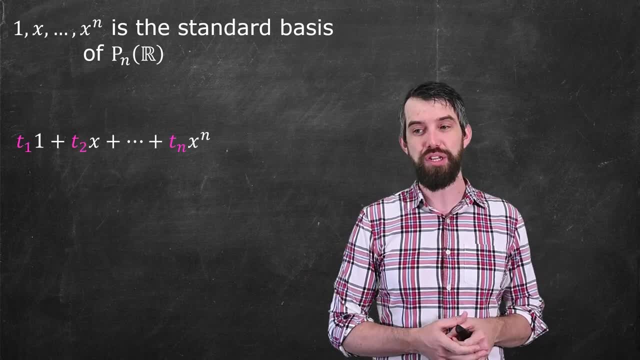 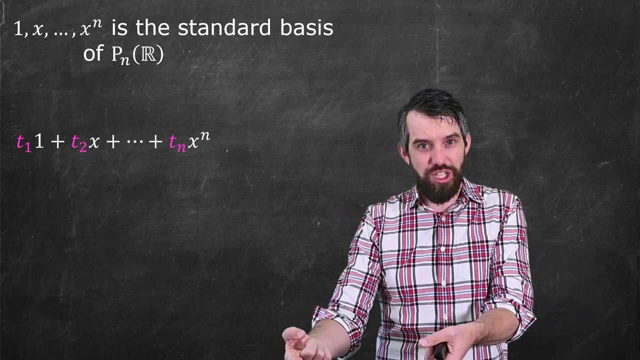 but just very, very briefly. if I look at the standard linear combination of these things, so a linear combination of the one down to the x to the n, then the corresponding coefficient matrix is just the identity matrix, the n by n identity matrix. 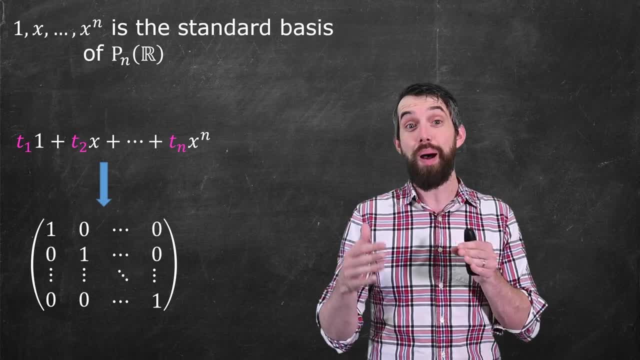 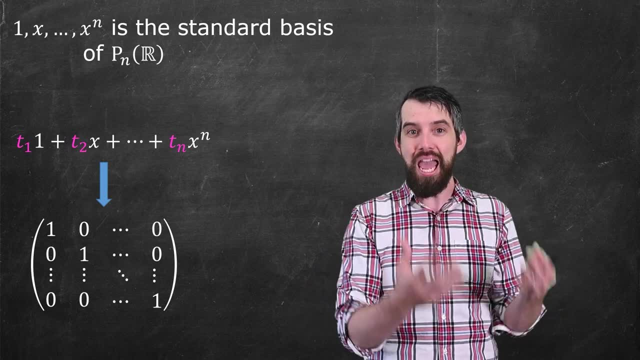 Note that this identity matrix is n plus one by n plus one. Indeed, when it was degree two or less polynomial, we had a third of it, a three by three matrix. So indeed, a degree n polynomial gives an n plus one by n plus one matrix. 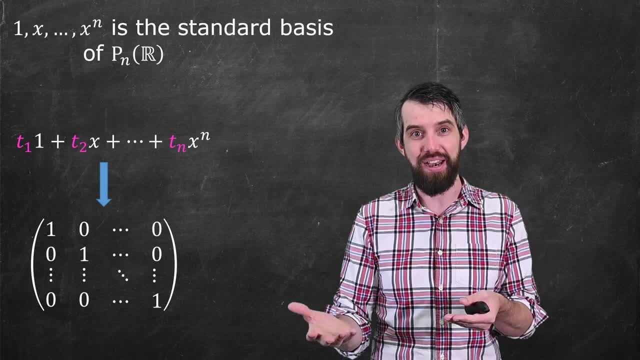 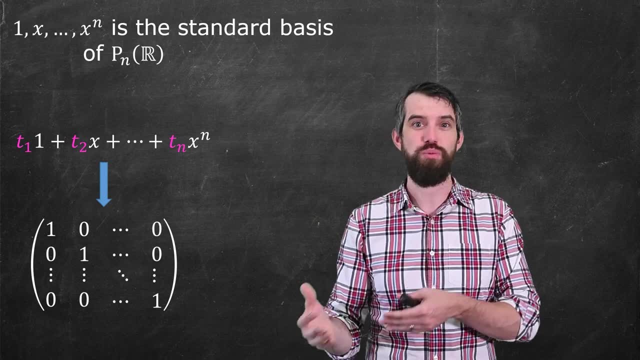 The basic reason here is that if you think about all the powers of n, we also have x to the zero being included, So it's going from zero up to n, and that's why there's n plus one of them. Either way, it's the identity matrix. 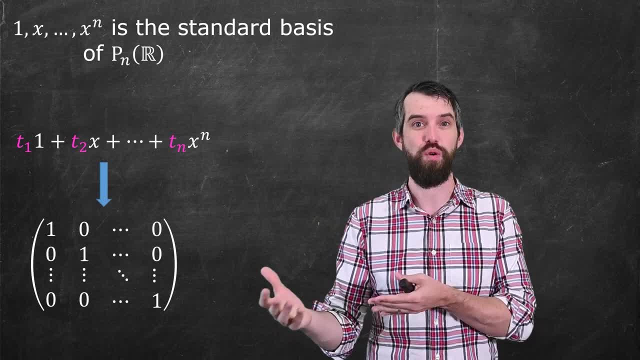 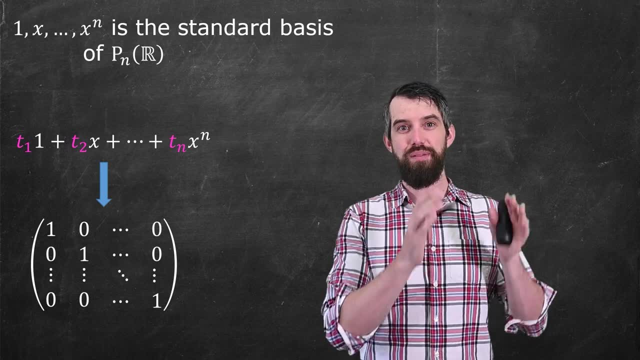 which has full rank and so has unique solutions to any system of equation. that's gonna give that it spans everything and that it's fundamentally independent. So, thinking about this vector space of polynomials, the parallels between what we studied before and what we're looking at now, 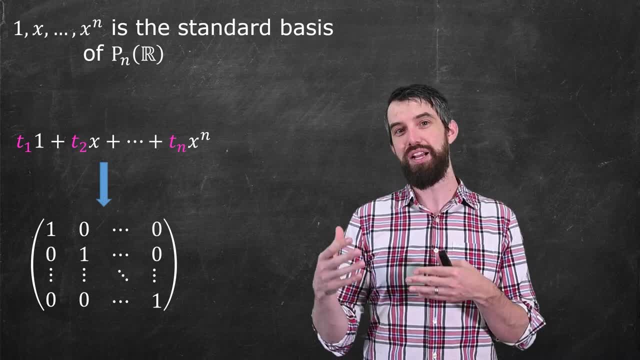 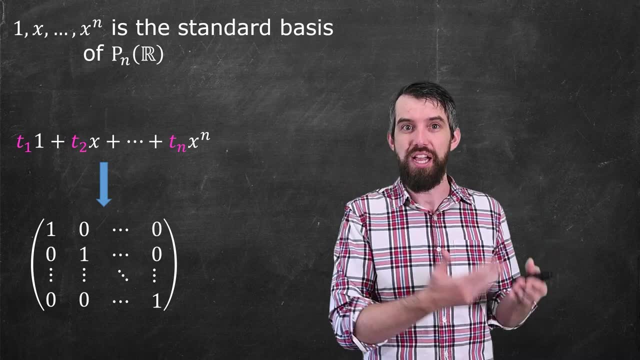 is really really very tight. Indeed, there's ways that you can actually think of polynomials of degree less than or equal to n as really just being the same thing, what we sometimes call isomorphic to the vector space: R, n plus one.